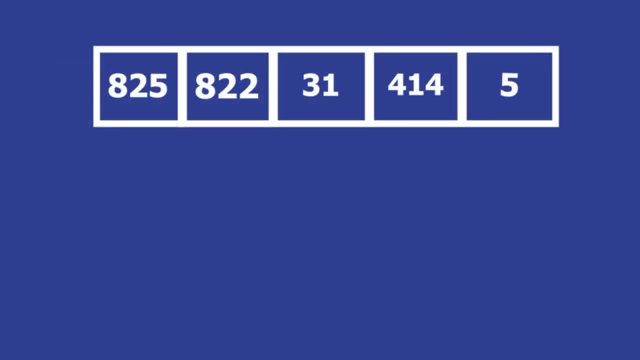 how and why that works. Here we've got our trusty RE again. First we're going to tackle the units places and we're going to have to calculate the frequency of each digit. There are 10 digits, from 0 to 9.. 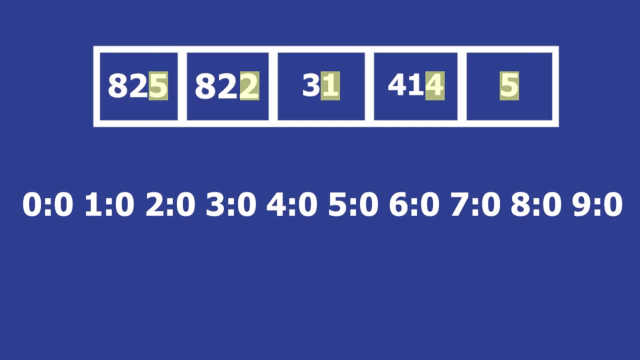 and we can see that 5 occurs twice. 5 is in the unit's place of 825 and 5 is in the unit's place of 5.. So the frequency of 5 is 2.. The unit's place of 822 is 2.. So the frequency 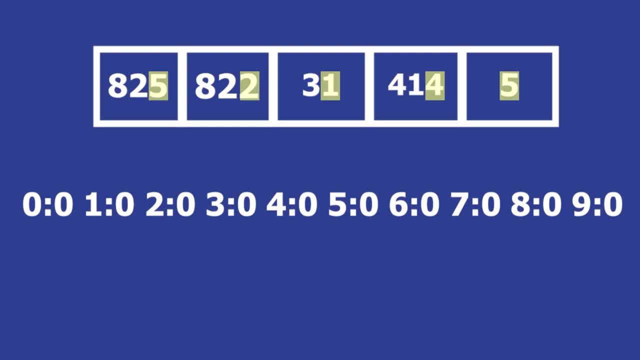 of 2 is 1.. The frequency of 1 is 1 and the frequency of 4 is 1.. What are these values supposed to tell us? They're supposed to tell us that 31 is the smallest number. It has the smallest unit's place at least, So it's supposed to go into the very first location. 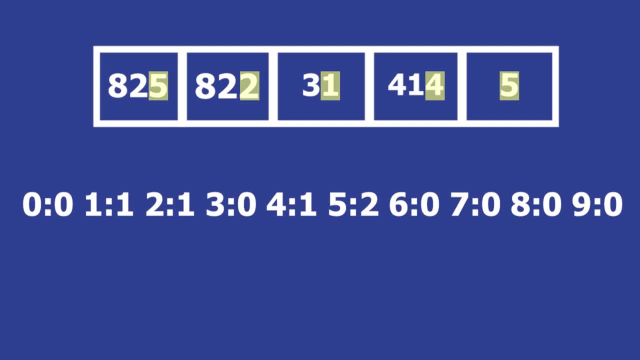 Then 822,. it has a unit's place of 2.. So it's supposed to go 1. after that, The number with a unit's place of 4, that is 414, has to be present after 822, and 825 and 5 are going. 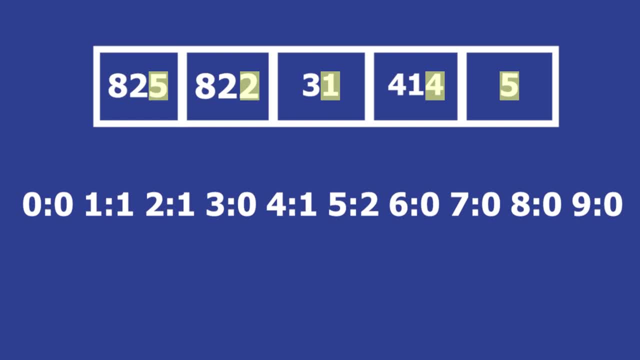 to have to occupy the next two places. That's why, in order to get the location values, we're going to add each number to its predecessor. Now we're going to add each number to its predecessor. Now, we're going to add each number to its predecessor. 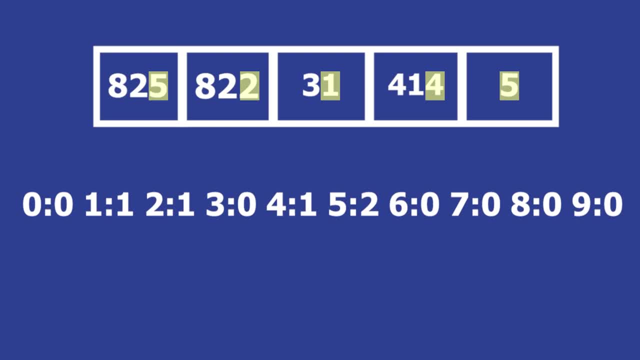 Now, 0 stays as 0. The number corresponding to 1 is going to become its value plus the previous value, that is, 1 plus 0, which is 1.. It stays as 1.. The number corresponding to 2 will be its value plus the previous value, 1 plus 1, which is 2, and we continue to do. 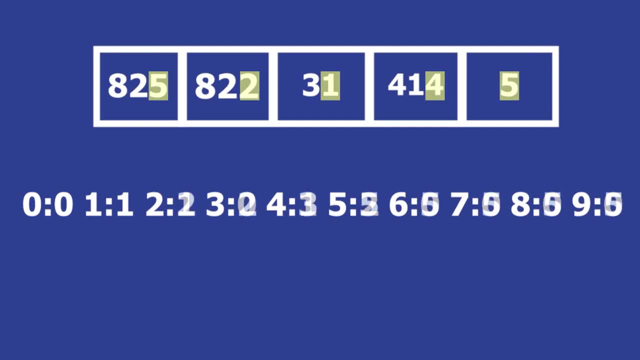 so for each and every number. This is the new location table which we get. What does this table tell us? We start a loop from the end to the beginning. Normally, we move from left to right. i is 0 to n-1.. Here we're going. 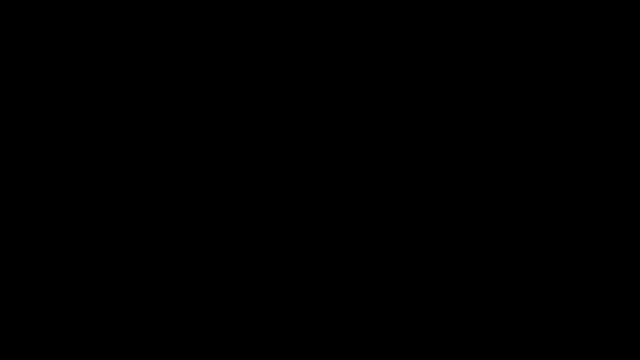 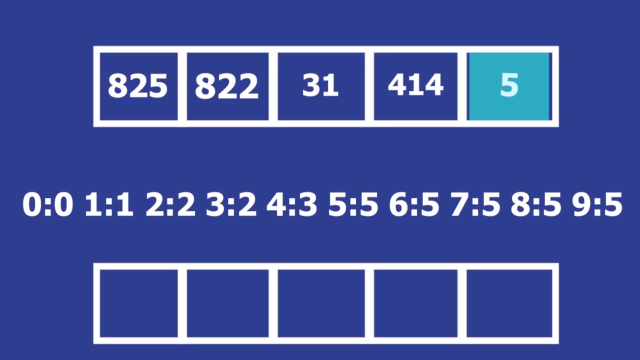 to move from n-1 to 0. Now why are we moving the loop from the end to the beginning? That will be understood in the next iteration. Now the unit's place at 5 is 5.. If we have a look at the location table, this tells us that that's going to occupy the 5th position. 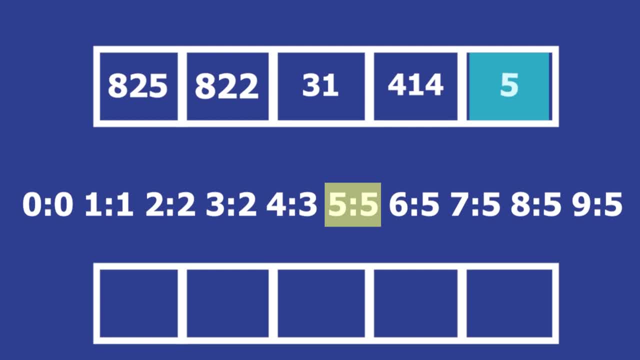 If it's 0 indexed, that's going to be position 4.. Let's just assume it's 1 indexed for convenience. 5 is going to be present. 5 is going to be present at location 5 in the final array. And now we've got to make. 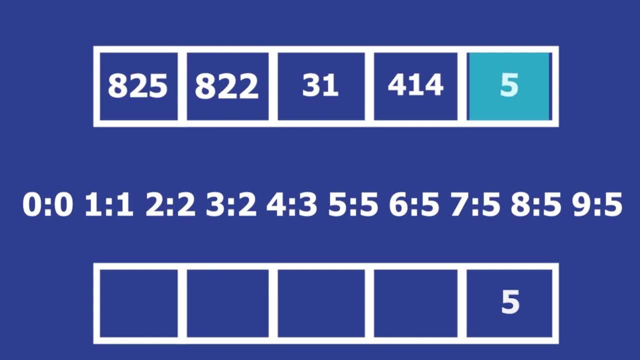 sure to decrement its location so that there's no overwriting. So the number corresponding to 5 becomes 4 and our loop moves down. The number corresponding to 4 is 3.. That tells us 414 is going to occupy the third position. Following this, we decrement its value and 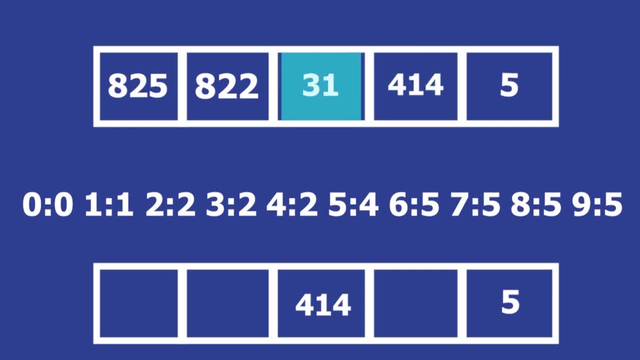 move our loop down: 31,. its unit's place is 1 and our table tells us that occupies the very first location. 31 goes into location 1.. We decrement its count and we have a look at 822.. Last digit, 2, it occupies the second location. Its count decreases and when we move to 825, we can. 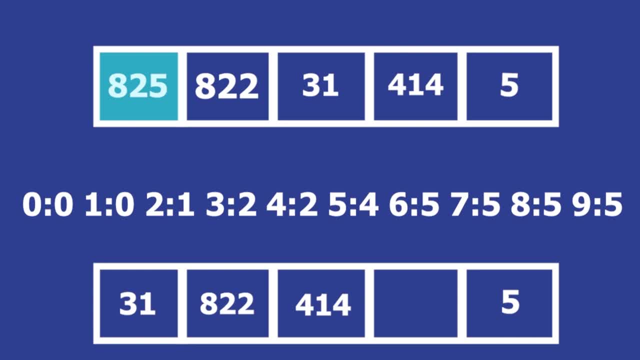 really see why it's so important to decrease the location value. If we had not done so, 825 would have overwritten 5 and we would have lost data. Since we decreased the value, 825 now goes into location 4.. This entire process is called counting sort. We've performed counting sort for the units. 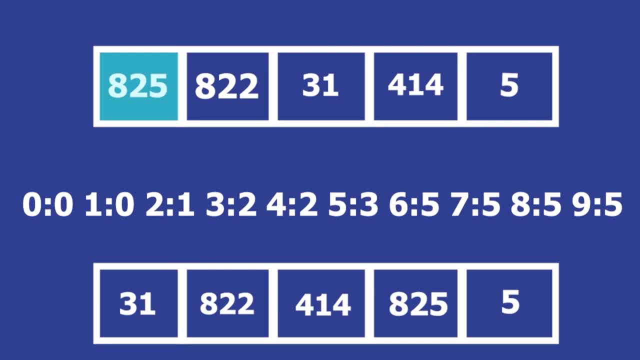 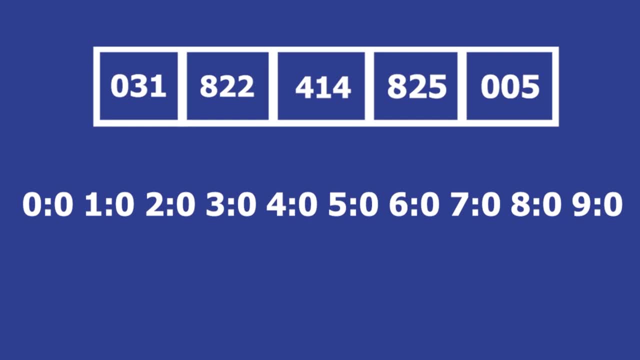 place. We have to perform it 2 more times for the 10th place and for the 100th place. Now we've got to count the frequency, the number of occurrences of each digit in the 10th place. Now you know the drill. We've got to add each value to its predecessor in order to 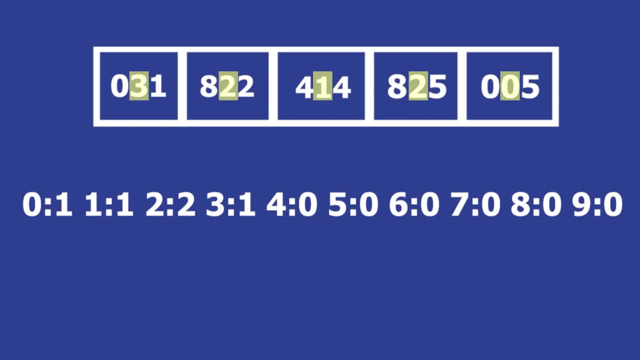 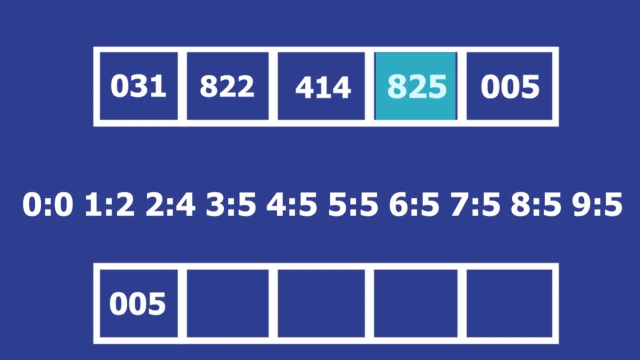 And here we see why it's so important to move from right to left. 825 and 822, they both have a 10th place of 2.. That means we're going to be visiting 2, 2 times Whenever we visit. 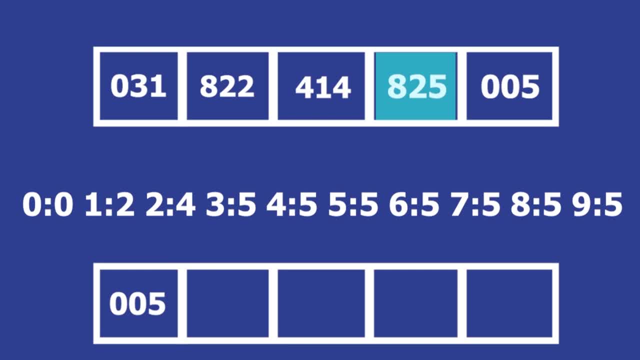 a number more than once. the number we visit first is going to occupy a later position, and the number we visit second will occupy an earlier position because, after we visit the number for the first time, we're going to decrement the count In order to ensure. 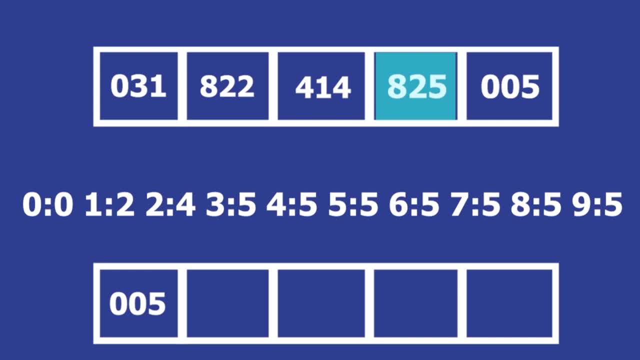 that 825 occurs after 822, we have to move from right to left, And after this iteration is done, the 10th places are going to be sorted, along with the units' places. After we place 825 into location 4, the value has to be decremented by 1.. now we 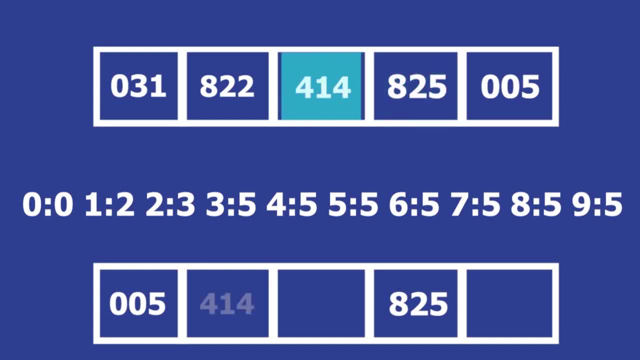 move on to 414.. It occupies the second position Once value decreases and 822 will occupy the third position. It will appear before 825.. 31 will appear at the end. If you ignore the hundreds places, you can see that the units places and the tens places. both have been 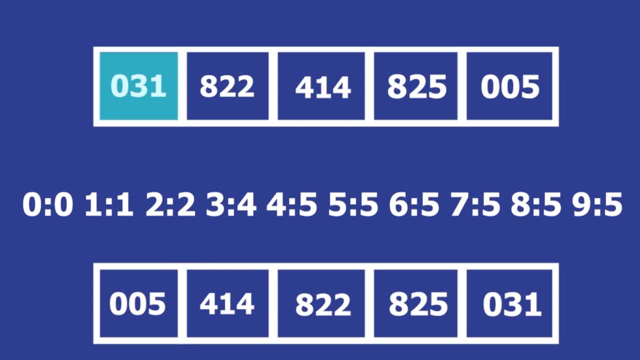 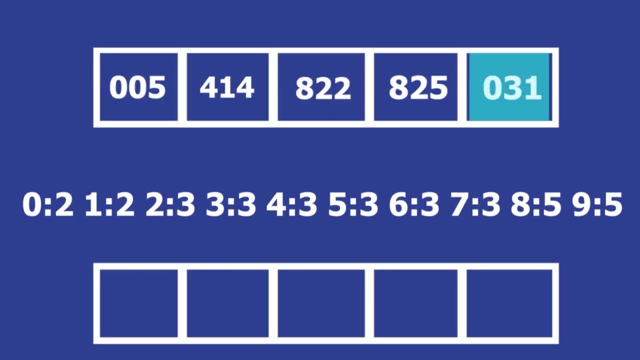 sorted. After each step, an additional place value gets sorted. This means that after the next step, the units, tens and hundreds places will all be sorted, meaning our entire array will be in increasing order. Now let's perform the final iteration a little quickly: 31 goes. 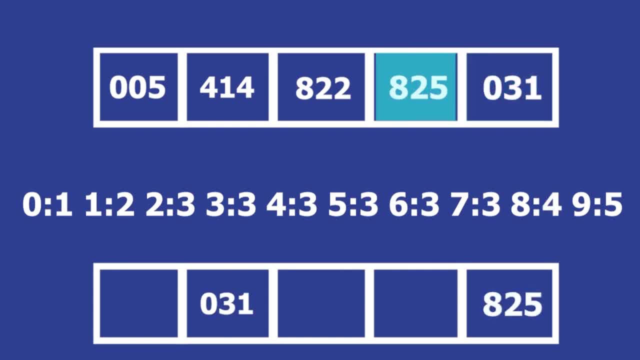 into location 2, 825 into location 5, 822 into location 4, since the location count has been decremented, 414 straight into the middle and 005 in the very beginning. Our array is now in increasing order. We performed n iterations for each step and how many steps are there? The total number: 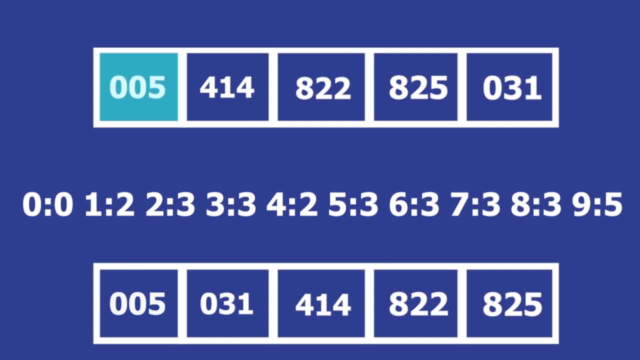 of steps is equal to the total number of digits in the maximum number. Here the max number is 822, which has 3 digits, which is why the total number of iterations is 3 into n. In general, the number of iterations will be k into n, where k is the number of digits in. 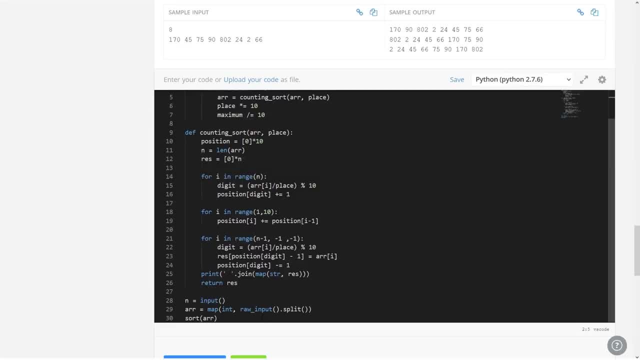 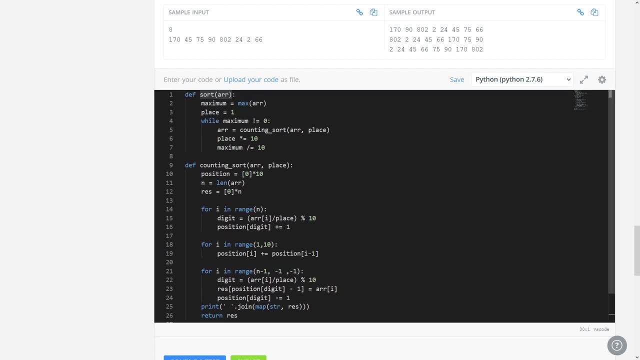 the maximum number. Let's have a look at the code. First we take the input and we sort it. The output of this sort function has to be a fully sorted array. In that sort function the first thing we do is identify the maximum number in the array, Say it has. 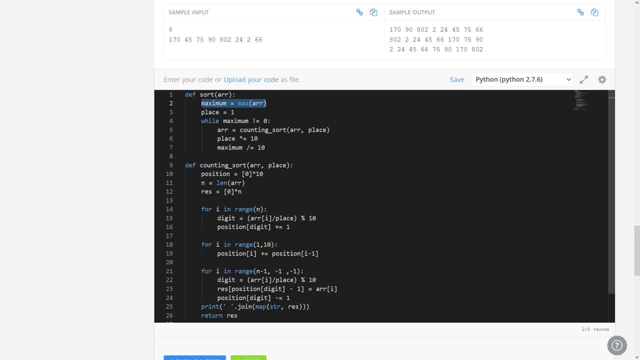 k digits we've got to ensure that we perform counting. sort k times Place will tell us the place value we're currently sorting. So initially we sort the units place, Then we multiply it by 10, indicating that in the next iteration we're going to sort the tens place. 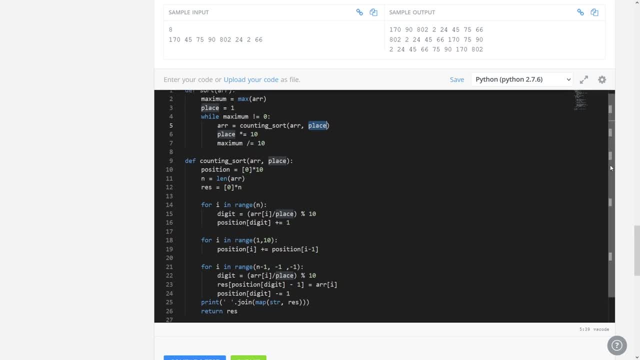 Then the hundreds place, and so on. As for the counting sort itself, this is where the bulk of our logic takes place. First, we're going to have a position array. It has digits from 0 to 9.. So a total of 10 digits. This for loop. what does it do? It identifies the 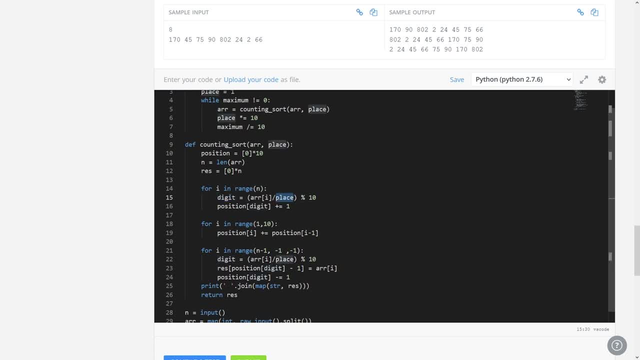 digit in that place. So initially, in the units place, we identify which digit is present and we increase its frequency. Following that, what we do is we identify its position by adding it to its previous value. Finally, let's just add an enter here. So finally, we run a loop from the end to the beginning, from n minus one. 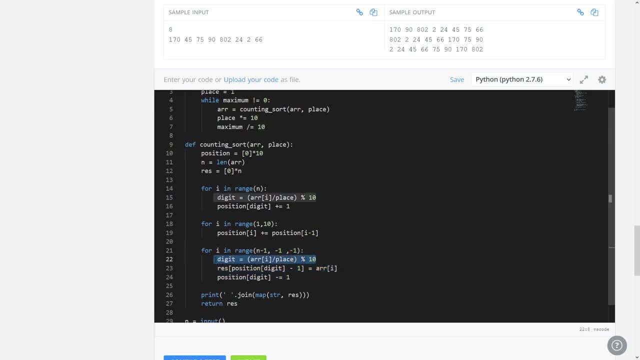 to zero. We identify digit because this tells us which location to look for in the position array. We go to that location. Remember that gives us a one indexed array. we have to make it zero indexed. So we subtract one and we place that element at that location in our 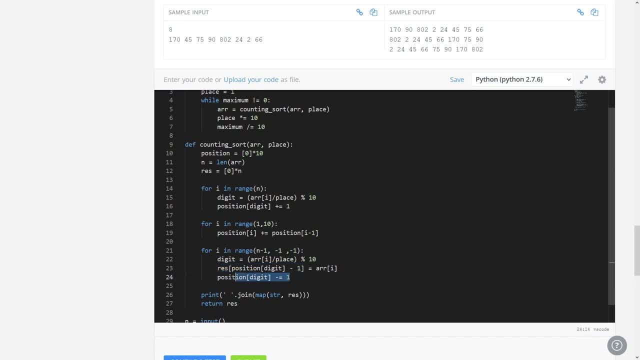 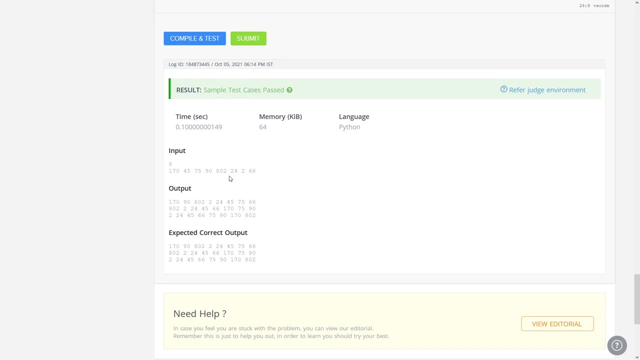 result array. And a very important step, don't forget, is to decrement position of digit by one, so as to prevent overwriting. Let's see if this works. Perfect, So you can forget the sample test cases part. essentially, what this program is telling us is, if this is our, 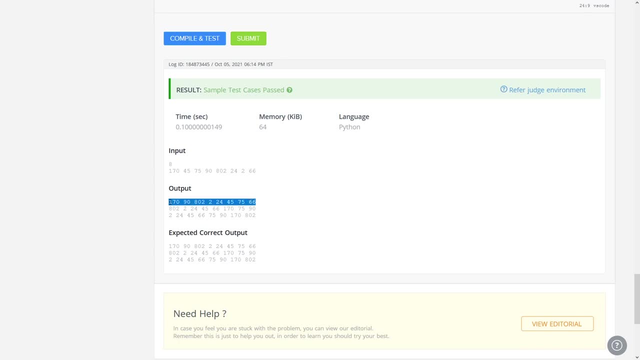 input array. After step one, this is going to be our output. after we sort the units place, After we sort the tens place, this will be our output. And after we sort the hundreds place, we will get a fully sorted array.